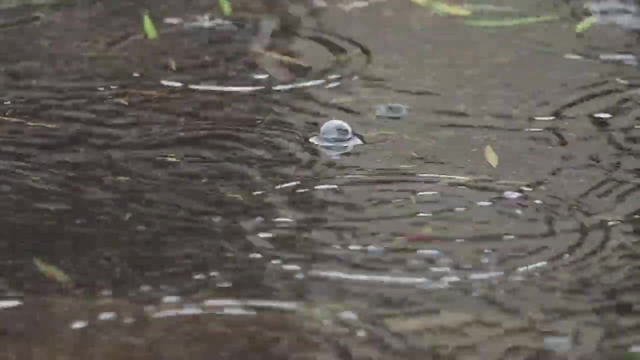 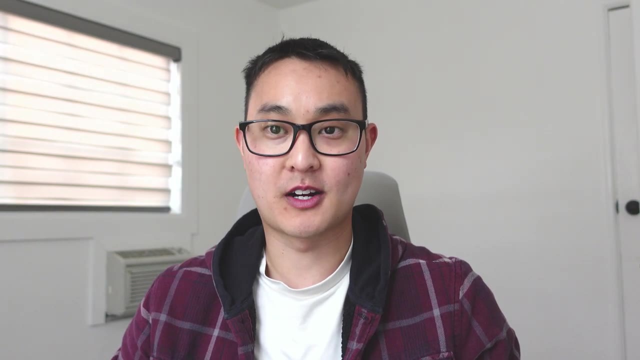 issues from managing water resources to designing systems to reduce air pollution. So here are some of the pros and cons to majoring in environmental engineering. Let's first start off with the pros of environmental engineering. The first one is the high demand for environmental engineers As more 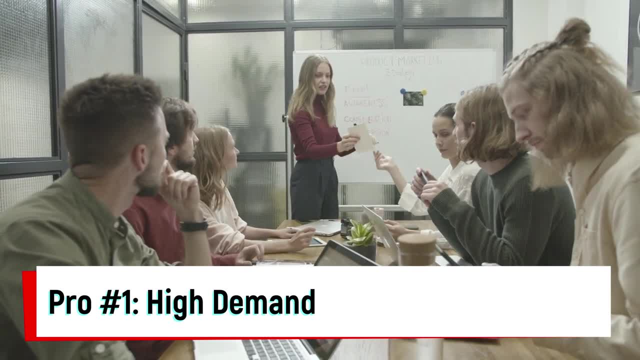 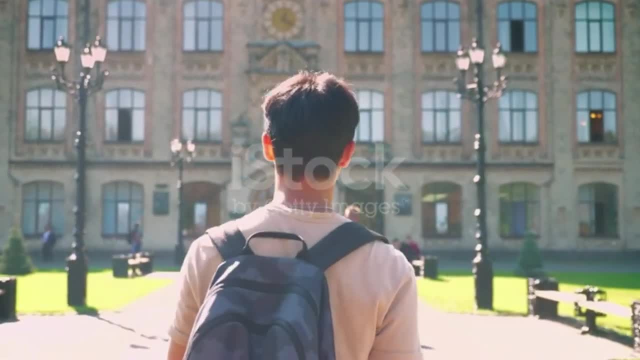 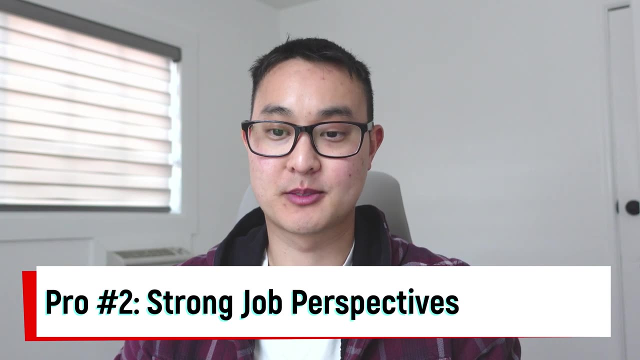 companies and governments seek to reduce their environmental impact, there is a growing demand for environmental engineers. This means that graduates of environmental engineering programs can expect to find job opportunities in a variety of industries, including engineering, construction and consulting. The second pro is strong job perspectives: Environmental engineers. 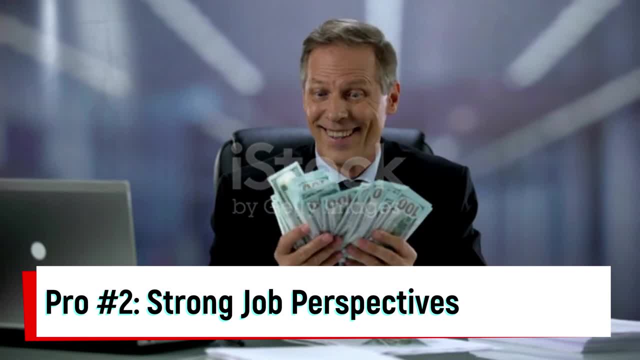 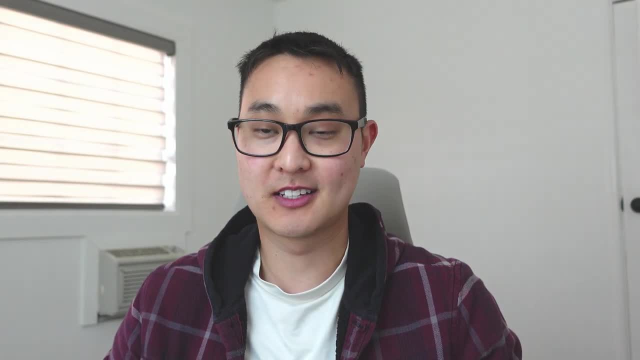 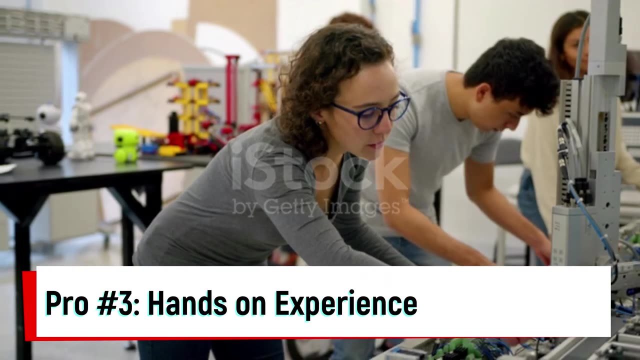 typically enjoy strong job perspectives, with a median annual salary of over $88,000 per year. I got this number off the internet. Each company can be different. don't expect that immediately for entry levels or even at your specific location. This is just an average. The third pro is hands on experience. Environmental engineering programs often include opportunities for hands on experience, such as internships, coops and research projects. 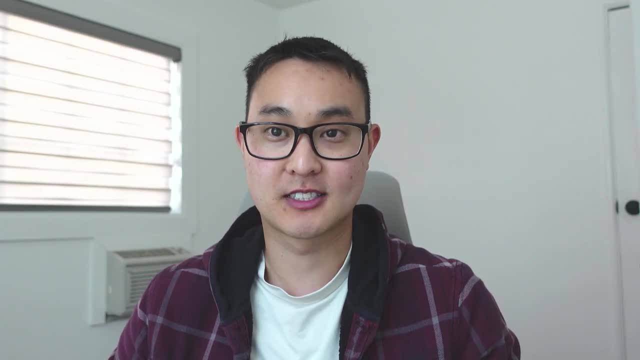 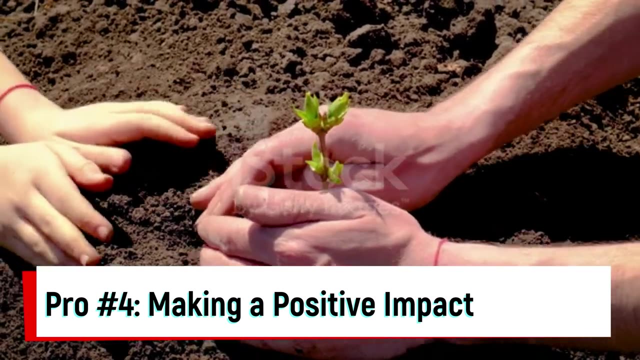 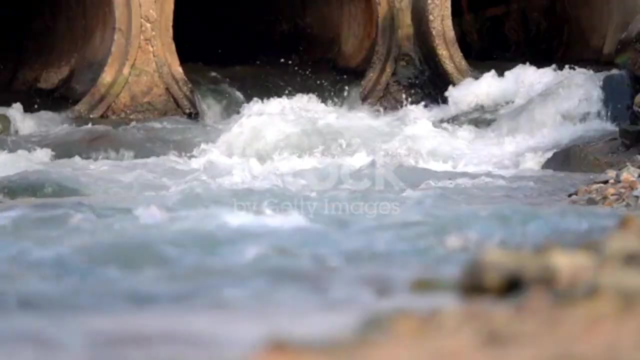 This can be a great way to gain practical experience and make connections in the field before your actual first job. The fourth pro to environmental engineering is making a positive impact, Although this could probably apply to both the environmental scientists. environmental engineers have the opportunity to work on projects that have a real impact on the environment, such as designing systems to reduce pollution or improve water quality. 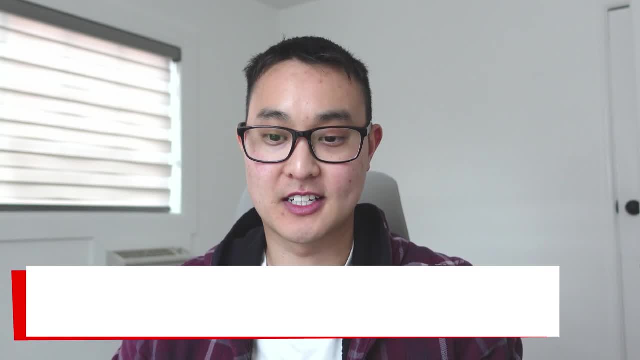 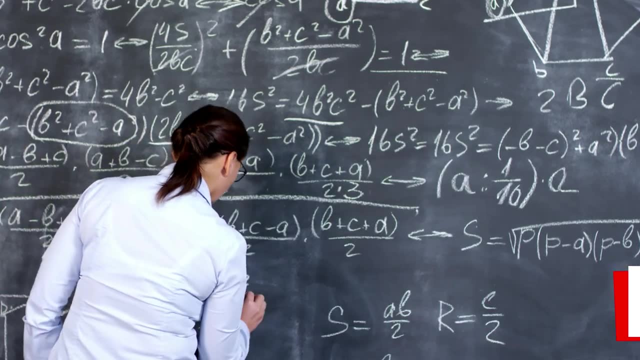 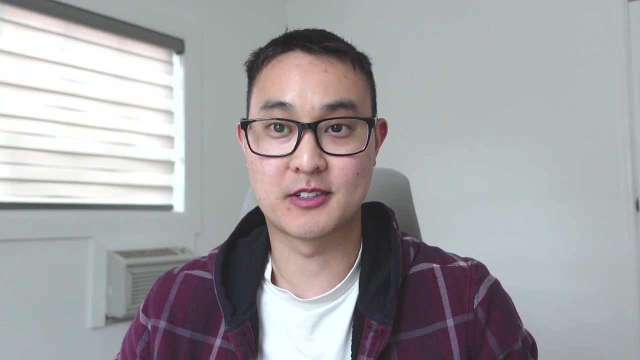 Now let's head to the cons of environmental engineering. The first downside is that there's heavy emphasis on math and science. Environmental engineering requires a strong foundation in math and science, including courses such as calculus, physics and chemistry. This can be especially challenging for students who struggle in these topics, so if you end up failing one of these classes, you might have to repeat them, or you just aren't cut out for the job. 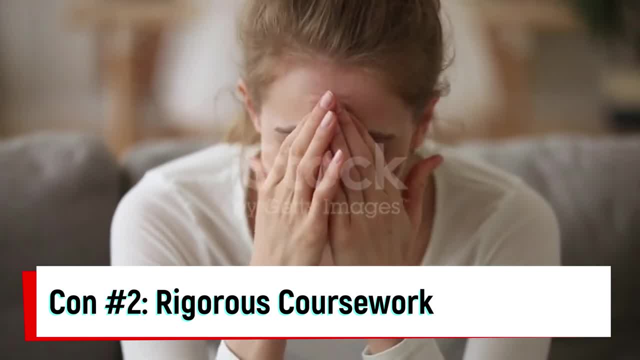 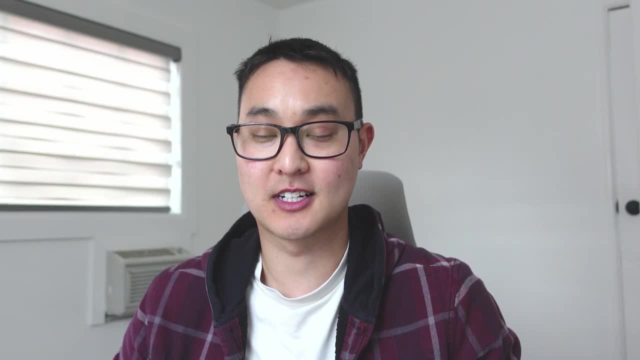 The second con is that there's rigorous coursework. Environmental engineering programs can be challenging and rigorous, with demanding coursework and high expectations for academic performance. So, going back to the heavy emphasis on math and science, it could be pretty hard, Even though you may want to major in environmental engineering. 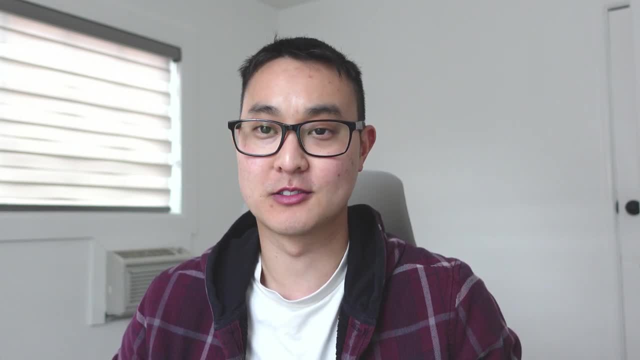 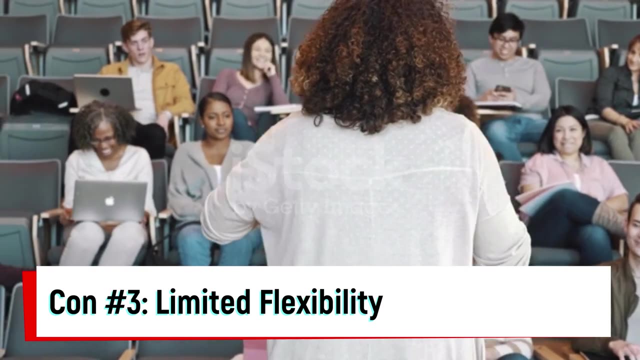 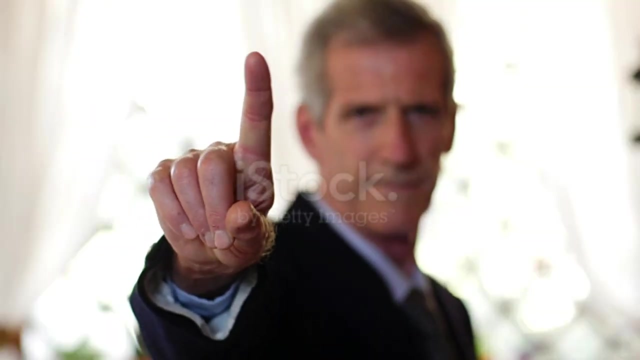 just the prerequisite courses and just not performing well in those classes could be your downfall. The third con is that there is somewhat limited flexibility. Environmental engineering programs tend to be more structured and less flexible than most other majors because it's pretty specific. This can make it difficult to pursue like a double major or to take elective courses outside of this major. 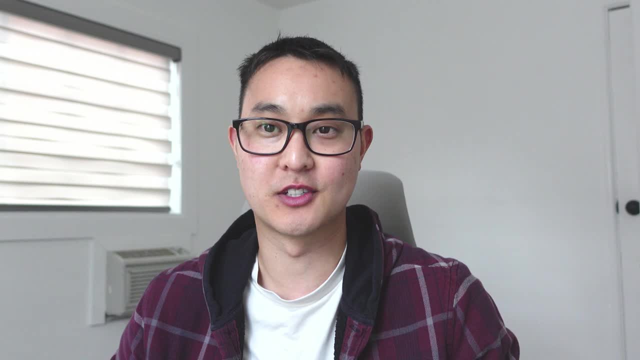 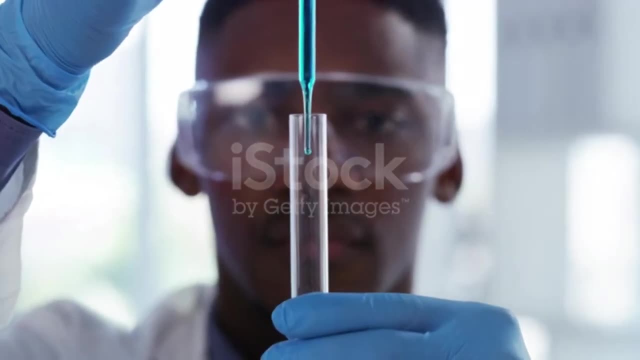 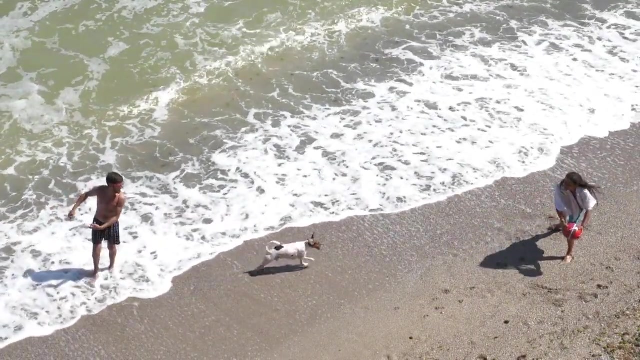 It's because, technically, environmental engineering is technically underneath the civil engineering umbrella. Now let's talk about environmental science. What is an environmental scientist? Environmental science- Environmental science is an interdisciplinary field that examines the natural world and how it interacts with human society. Environmental science majors study a wide range of topics, including ecology, geology and climate science. 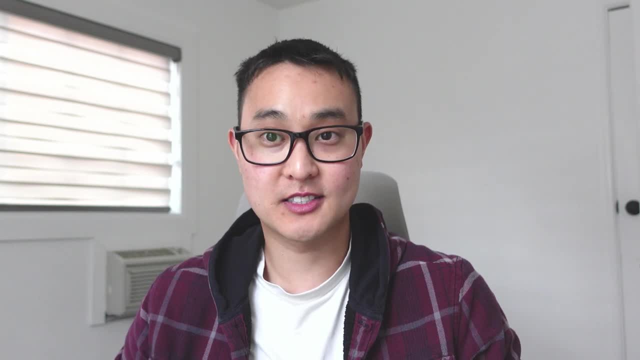 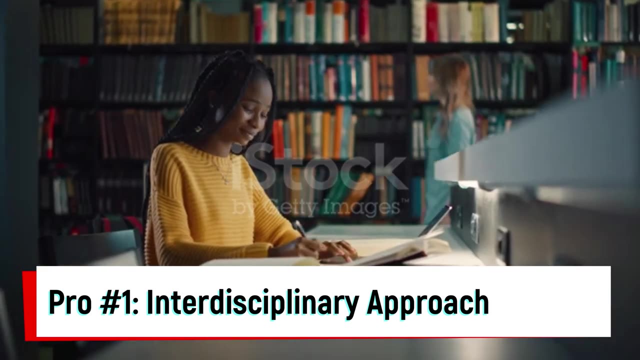 So here's some pros and cons to majoring in environmental science. Let's start off with the pros first. The first pro to environmental science is that it's an interdisciplinary approach. Environmental science is an interdisciplinary field, which means that students have the opportunity to explore a wide range of topics and different approaches. So it's not as limited as Environmental Engineering. The 2nd pro is that it's pretty flexible. Environmental science programs tend to be more flexible than environmental engineering programs, With more opportunities for students to choose elective courses and explore different areas of interest outside of environmental science. 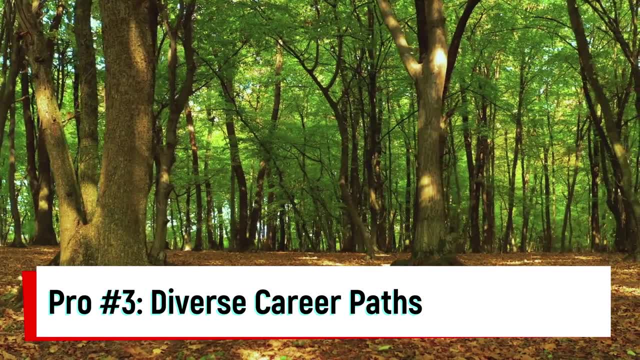 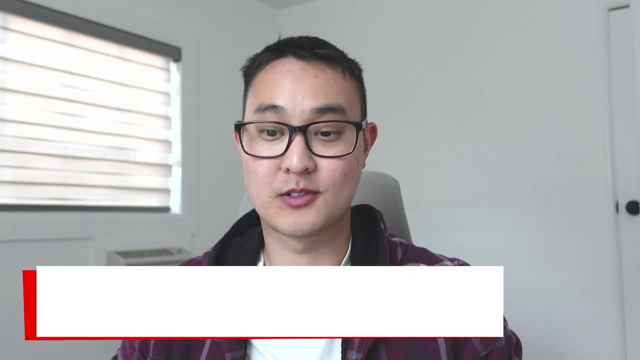 The 3rd pro is that it has a pretty diverse career path. Environmental science majors can pursue a wide range of career paths, including conservation policy, research and education. The 4th pro is that it has some hands on experience as well. 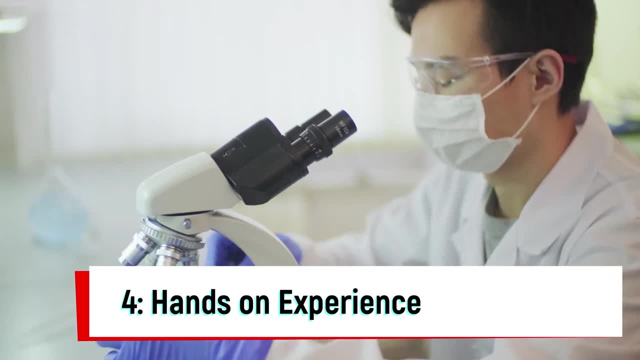 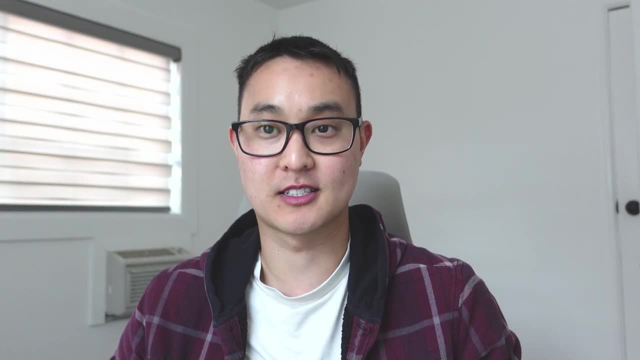 Many environmental science programs include opportunities for hands-on experience, such as internships and research projects- Pretty much the same pro as environmental engineering, and this can be a great way to gain practical experience and make connections in the field before your first entry-level job. So now let's talk about the cons of environmental science. The first and 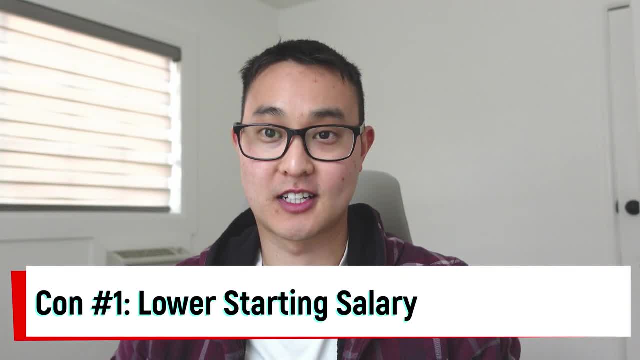 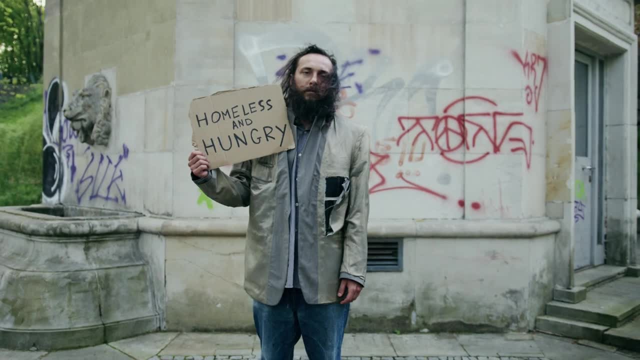 probably the largest con out here is that it has a lower starting salary. Environmental science majors tend to earn a lower starting salary than environmental engineering majors, with a median salary starting at around 50,000 US dollars per year. Again, it's just an average, but for the most. 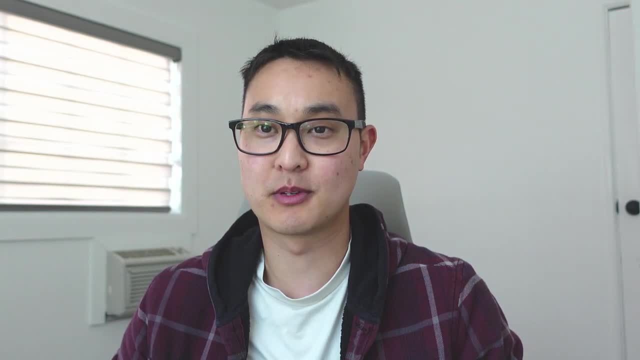 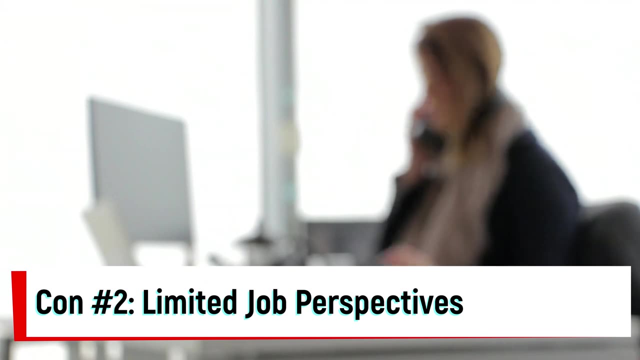 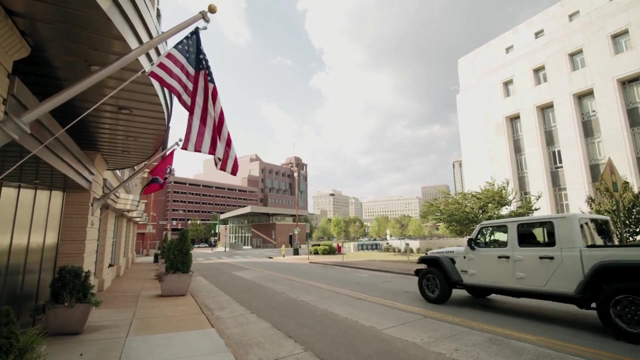 part. in general, environmental scientists do typically tend to get paid less than environmental engineers. The second con is that there is limited job perspectives. While there is a growing demand for environmental scientists, job perspectives can be limited compared to environmental engineering. Many environmental science positions are in government, education and non-profit sectors. 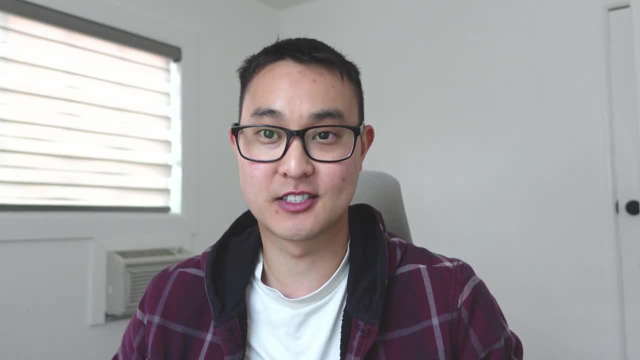 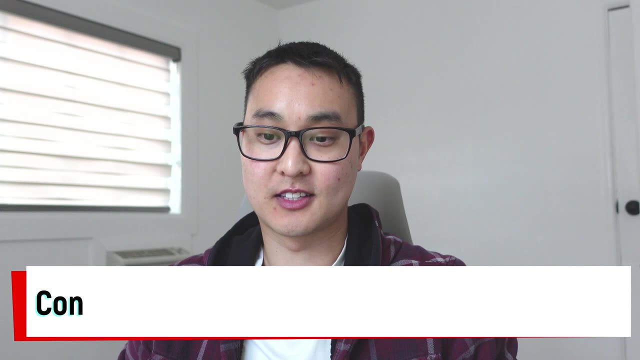 So if you do know anything about those fields, it is pretty hard to get in initially, Like if you have no connections at all or no work experience. then it's nearly impossible to get your foot in the door. The third con is that there is limited job security Environmental. 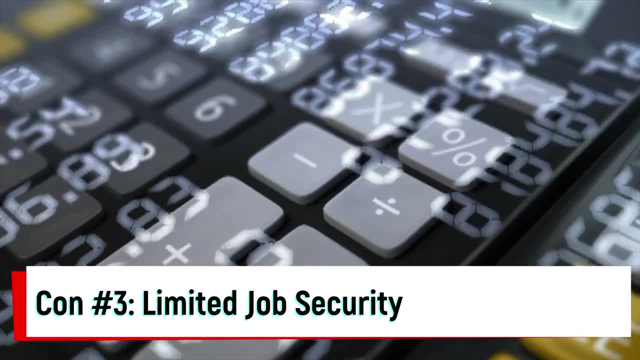 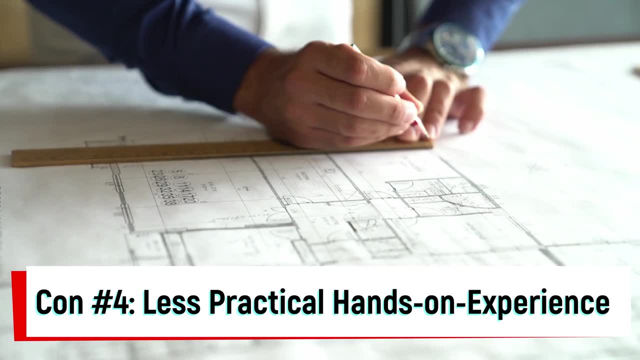 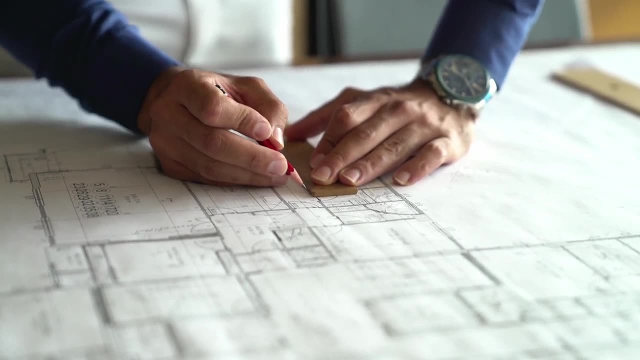 science jobs can be subject to funding cuts and other uncertainties, particularly in the government and non-profit sectors. The fourth con is that there is less hands-on experience. While environmental science programs often include opportunities for hands-on experience, they may not provide the same level of practical skills and technical training as environmental engineers. So the question is: